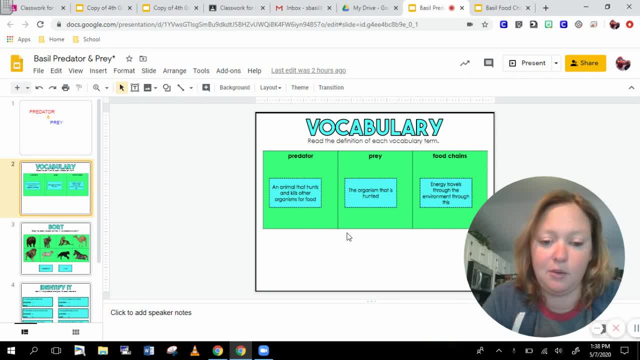 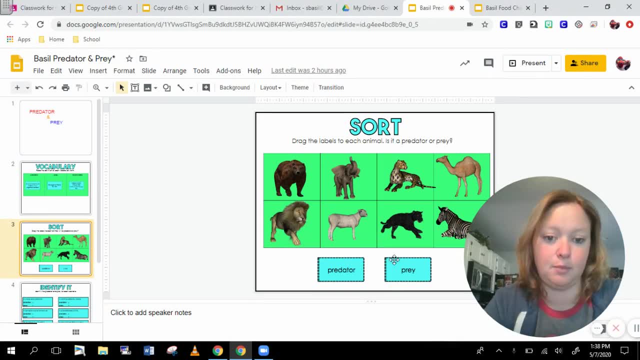 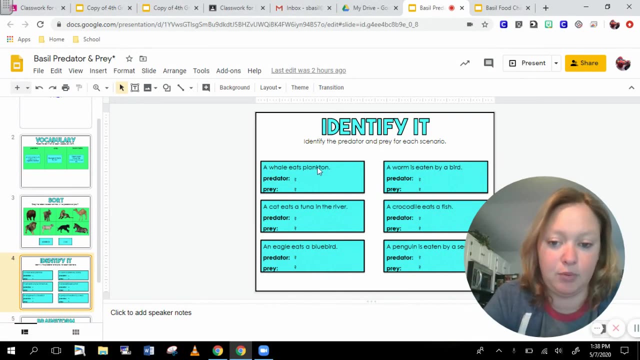 Predator and prey. So you have the definition. So you just need to read them And then you have a sort. So you have to drag the labels. If it's a predator, click predator and drag it prey. So far simple there. Identify what a whale eats plankton. Which one is the predator? So is the. 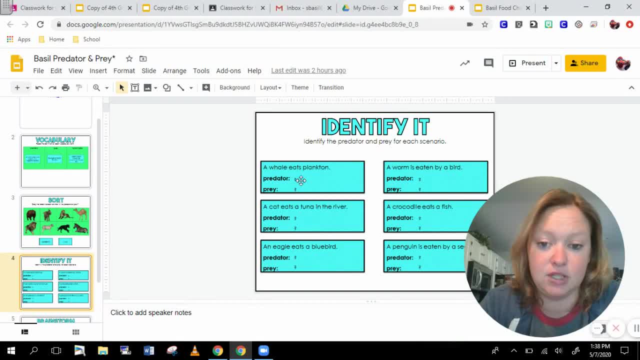 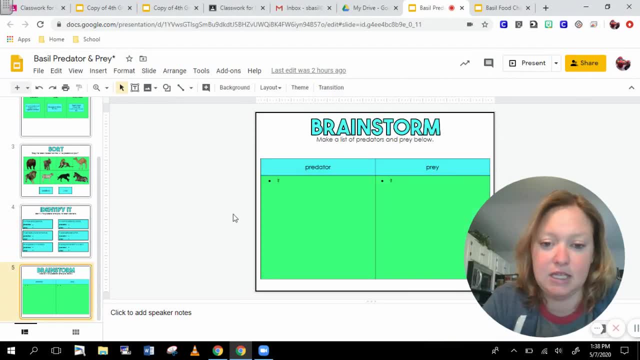 whale the predator, or the plankton the predator, Which one's the prey? So you would click and then you would type it in there And then the last one on this slide is make a list of predators and preys that you know. I would definitely probably use the information from slide four to complete. 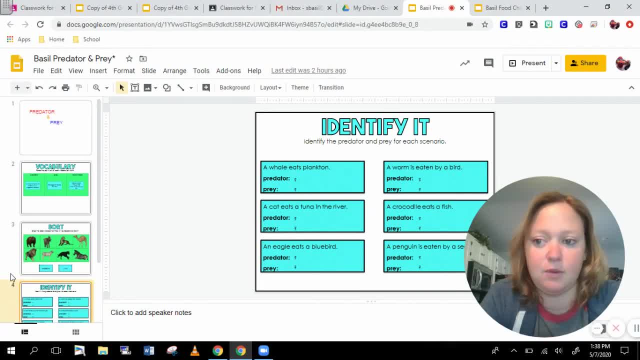 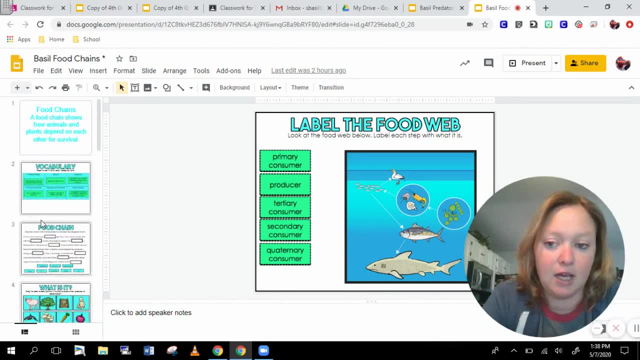 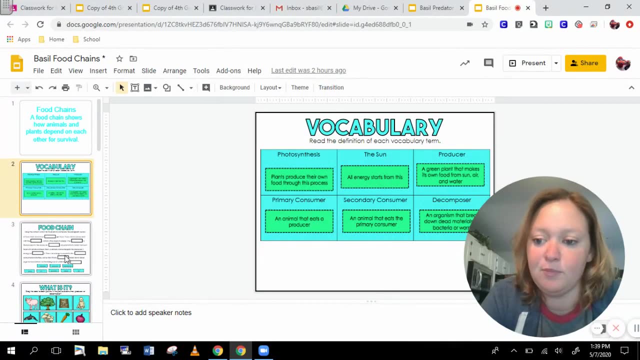 slide five. That's it for this, The first one. So predator and prey. And then you have a food chain assignment that you need to do. So you have the vocabulary- I definitely suggest reading over the vocabulary here- And then you have a fill in the blank. So you're going to click it and drag it and move it where. 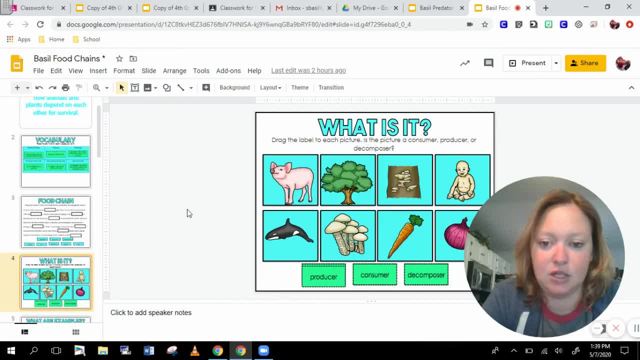 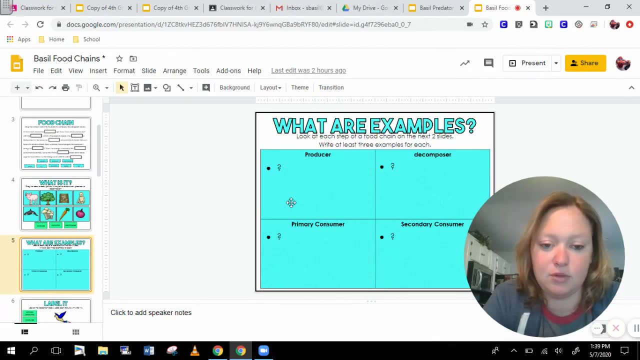 it needs to go. And what is this? So drag the label of each picture And then what it is. So is this a producer or consumer or decomposer? And then you'll click it and drag it. What are examples of producers, decomposers, primary. 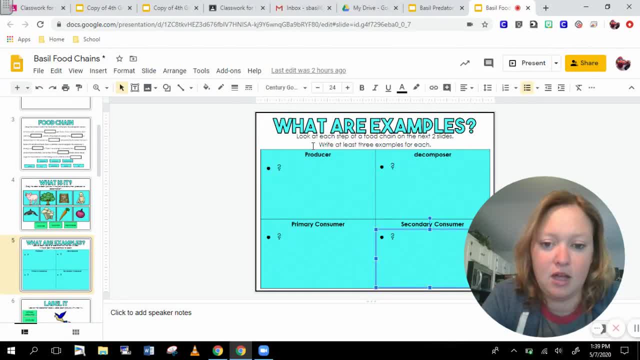 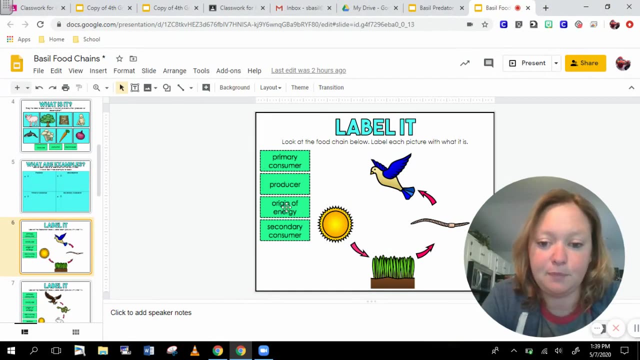 consumers and secondary consumers. So look you, look at, let's say look at- each step of the food chain in the next two slides and then write down three. So using the next slides, you can use those for those examples. Here you're going to label it with the origin of the energy. So where's all? 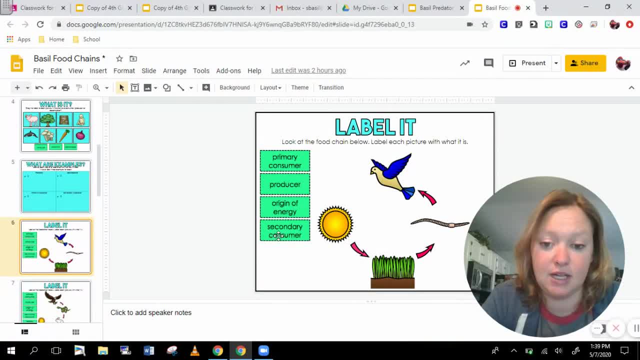 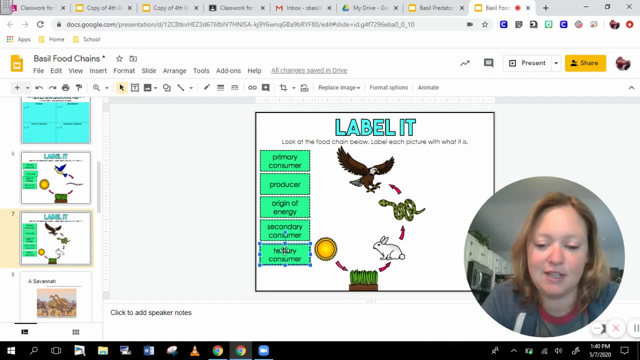 the energy coming from? What's the the producer, what's the primary consumer and then what's the secondary consumers? you'll drag and kind of move it to label the different things on that slide. same with this, but you have a new word: territory. I'm pretty sure it's how you. 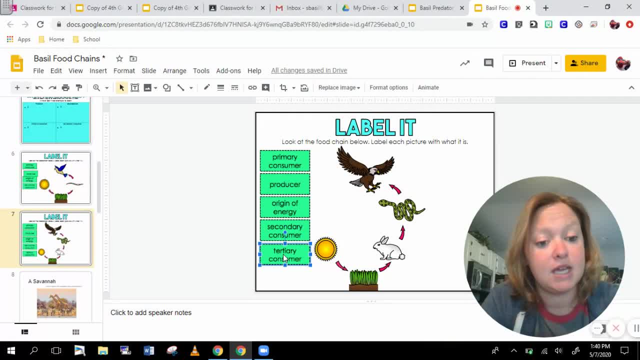 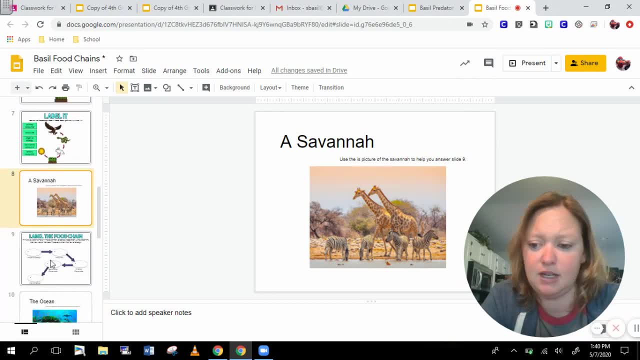 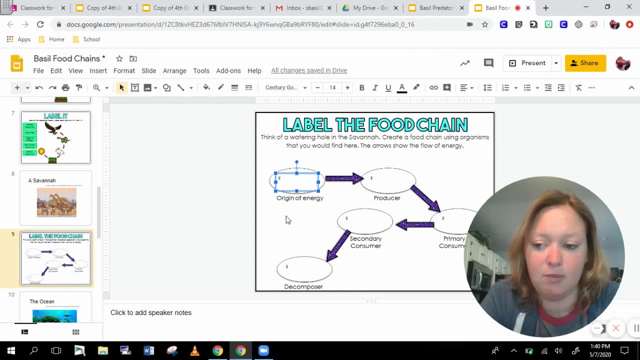 say it. so that's the top of your food chain. so whatever animal is kind of the top of your food chain, then use this picture of the Spanish. help you answer slide 9. so you need to label where the energy is coming from. it's gonna be the.